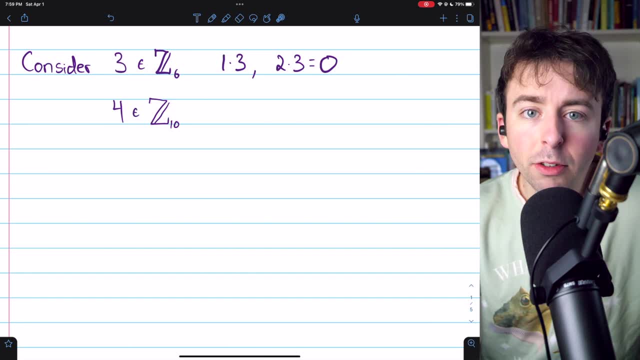 So what we see is that 2 is the smallest positive integer n, so that n times 3 is equal to the identity. The smallest integer satisfying that equation, positive integer anyway, is 2. And so we say that the order of 3 in this group, which we could also denote like this with magnitude bars, is equal to 2. In the same logic, we could figure out what the order of 4 is as an element of the additive group of integers mod 10. 1 times 4 is just 4, 2 times 4 is 8, 3 times 4 is 2, and 3 times 4 is 6. And 7 times 4 is 8, and 7 times 4 is 6. 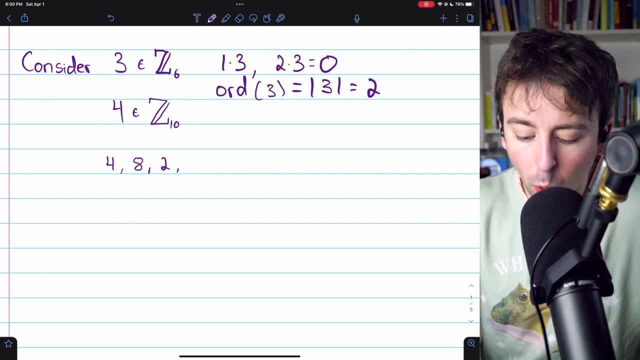 12, which is 2 mod 10. 4 times 4 would give us 16, which is 6 mod 10. And then 5 times 4 is 20, which is 0 mod 10. And so, we see, what is the smallest positive integer n, so that n times 4 is the identity of this group? Well, the smallest such integer is 5. That's the smallest positive integer that, when multiplied by 4, gives us the identity of the group. 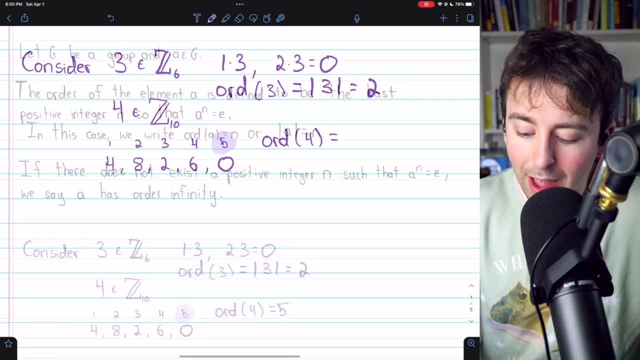 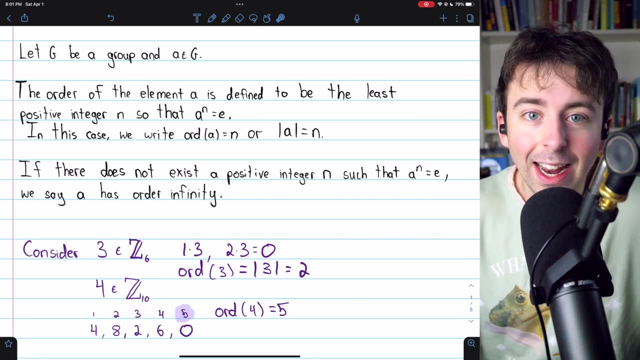 And so, we say the order of 4 is equal to 5. Alright, here's the definition. And the definition is written in multiplicative notation, although the examples we saw were in additive notation. Let g be a group and a an element of g. Then we say that the order of the element 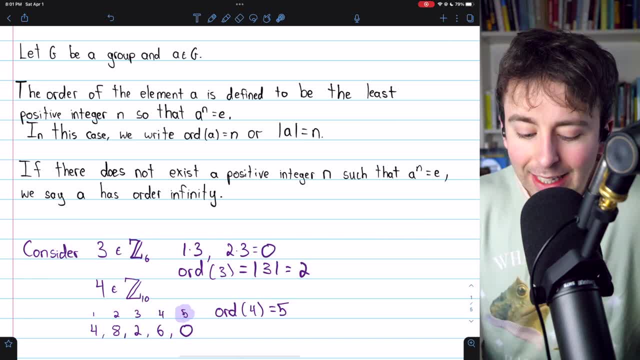 a in the group g is defined to be the least positive integer n, so that a to the n equals e. If we were using additive notation, then we would write this part as the smallest positive integer n, so that n times a is equal to e. And of course, we're assuming that e is the identity of the group. So, it's the least positive integer n, so that a to 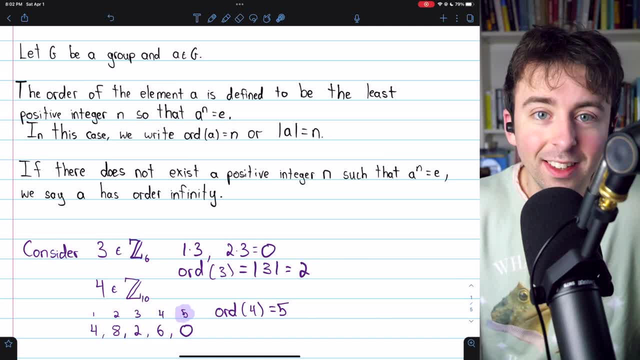 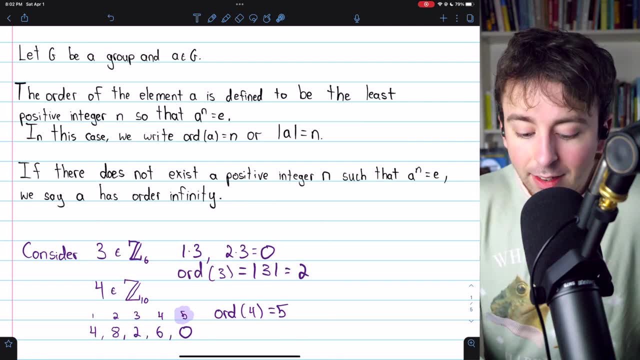 the n is the identity of the group. That's what the order of a is. And in this case, we write that like this, or with the magnitude bars like we saw before. Now, certainly, such an integer is not always guaranteed to exist. There's not always going to be a positive integer solution to this equation in every group. 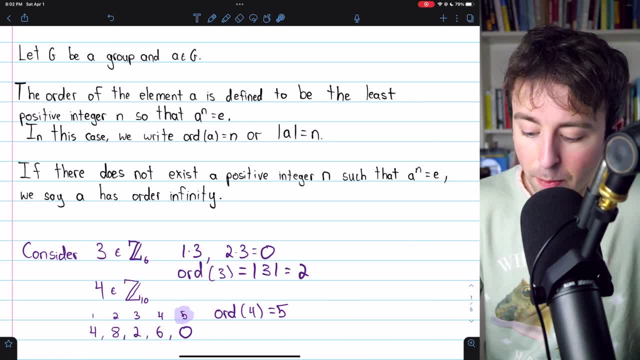 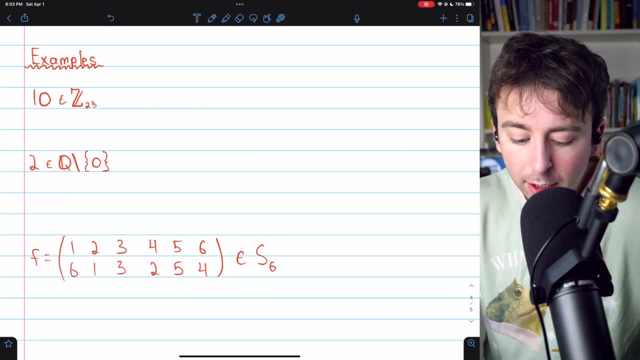 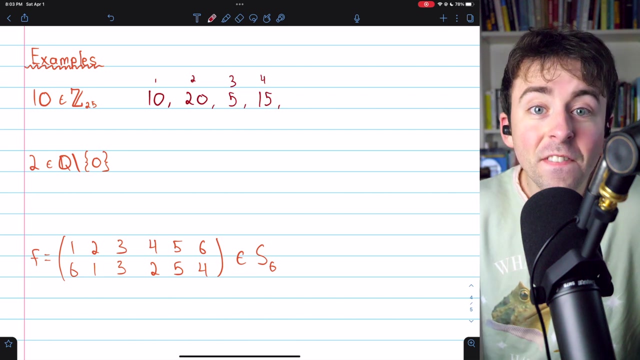 And if there doesn't exist such a positive integer, then we say that the element has order infinity. Let's finish with a few more examples. Let's begin with 10 as an element of the additive group of integers mod 25. So, we're back to additive notation here. In this case, 1 times 10 is just 10. And 2 times 10 is 20. 3 times 10 is 30, which is 5 mod 25. And then 4 times 10 is 40, which is 15 mod 25. And then finally, 5 times 10 is 50, which is 0 mod 25. So, the smallest positive integer n, so that n times 10 is the identity of the group, turns out to be 5. And so, we could write that the order of 10 in this group is equal to 5. Now, let's consider 2 as an element of the additive group of the multiplicative group of rationals without 0. So, this is a group since every element has a multiplicative inverse because we've excluded 0. If we just consider 2 to the 1, that, of course, is just 2. Then 2 to the 2 is 4. And then 2 to the 3 is 8. And then 16. And so on. Looks like we're never going to get back to 1, are we? Certainly not. 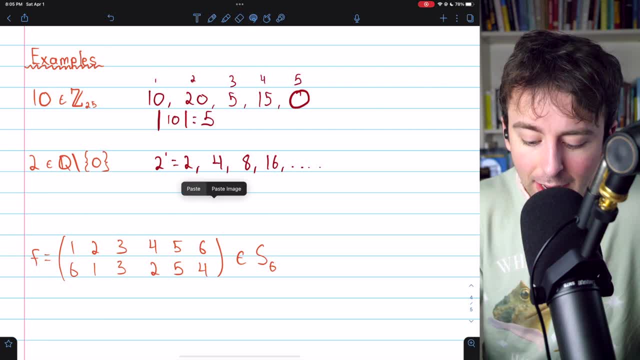 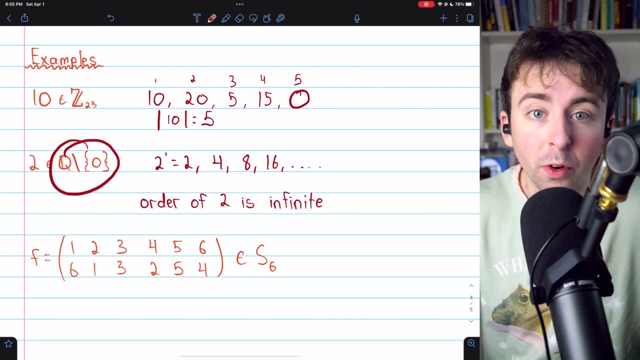 So, in fact, the order of 2 in this group is 1. And then 2 to the 2 is 4. And then 2 to the 3 is 8. And then 16. And so on. Looks like we're never going to get back to 1, are we? Certainly not. So, in fact, the order of 2 in this group is infinite. There's no positive integer n, so that 2 to the n is equal to the identity. The identity of this group, of course, is 1. So, again, no positive solution to this equation. And thus, the order 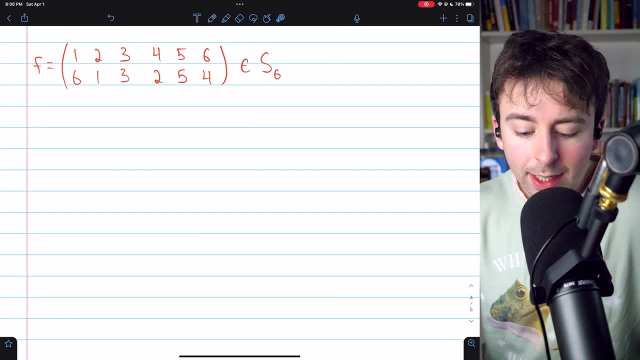 of 2 is infinite in this group. Finally, let's consider this permutation f from the symmetric group on six elements. I'll leave a link in the description to my lesson introducing permutations and the symmetric groups if you need a recap. But what this notation means is the function f is a permutation on a set of six objects. And what it does is it sends the first object to the sixth. It sends the second to the first, the third to the third, and so on. Now, the operation in this group, the symmetric group on six elements, is function composition. 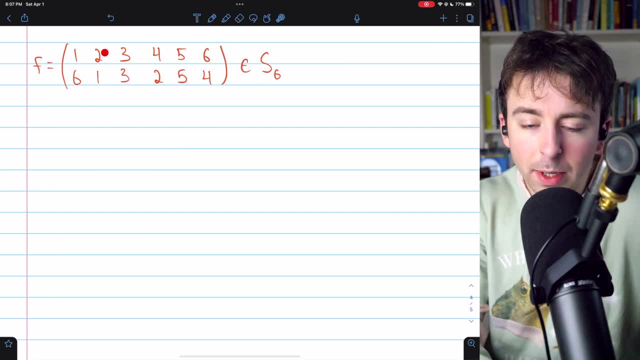 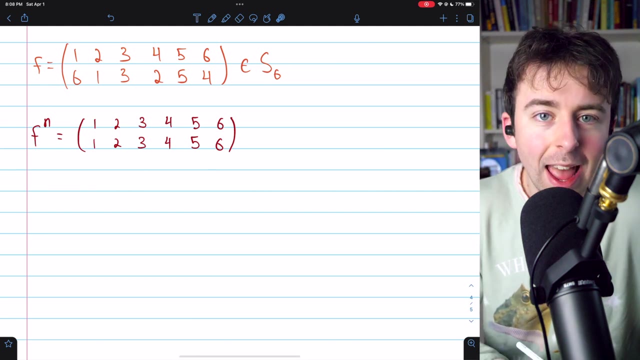 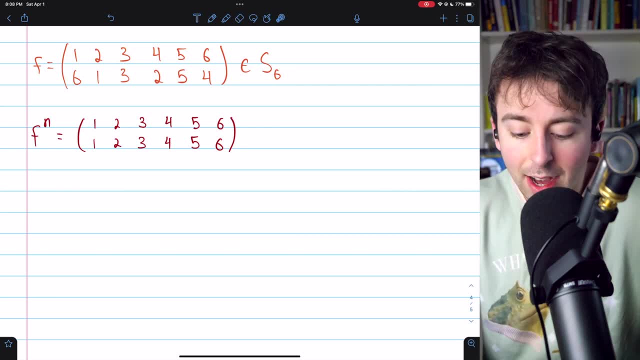 A third application, so f to the 3, would then send that 4 to 2. The net effect would be sending 1 to 2 in that case. And then finally, a fourth application of f, so f to the 4, would take 1, send it to 6, which would then get sent to 4, which would then get sent to 2, and then back to 1. 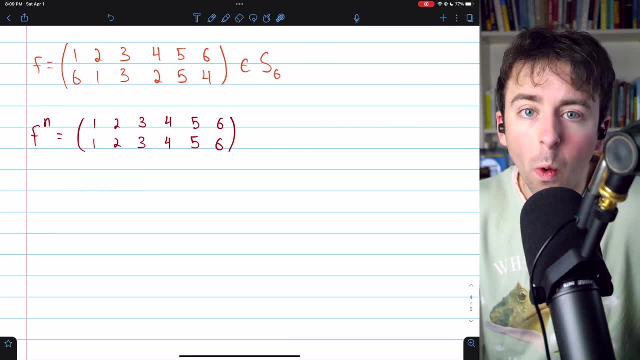 Meaning the net effect of f to the 4 is to send 1 back to itself. I'm not going to go through all the details here, but you can work out for yourself that indeed f to the 4 has this effect on every element. It sends each of 1 through 6 back to themselves. 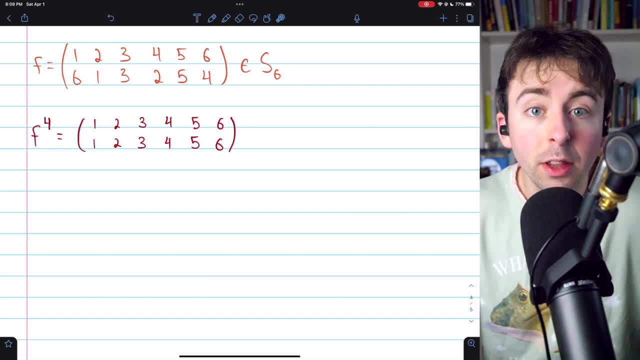 For one more example, let's consider 6. So we've got f to the 4. What's that going to do to the element 6? The first application of f would send 6 to 4. 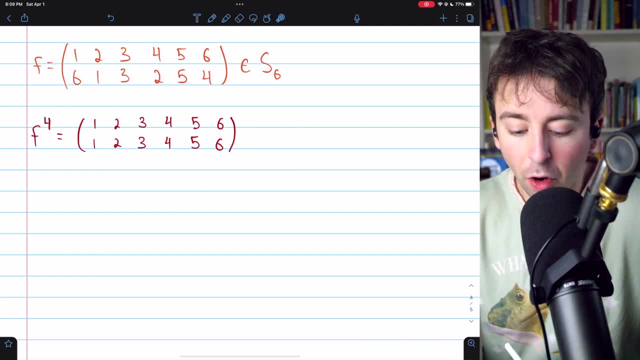 The second would send 4 to 2. The third application would send 2 to 1. And then the fourth application would send 1 back to 6, the net result being that 6 got mapped to itself. 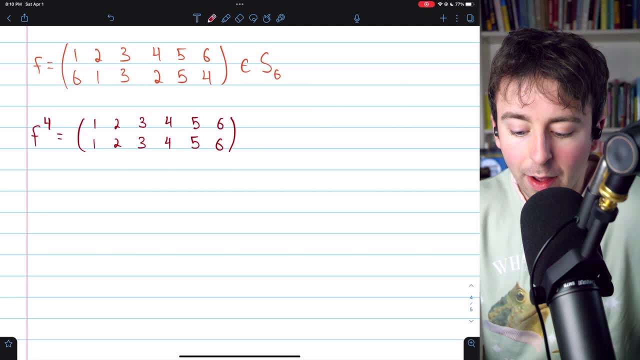 Since 4 is the smallest positive integer such that f to the 4 is equal to the identity, we can say that the order of this permutation f in the symmetric group S6 is equal to 4. Let's just mention two important theorems. Let's just mention two important theorems. 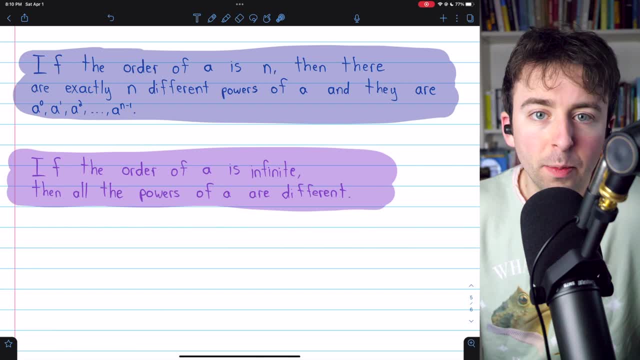 matters regarding the orders of elements before we go, I'll leave links in the description to my lessons proving these two theorems.